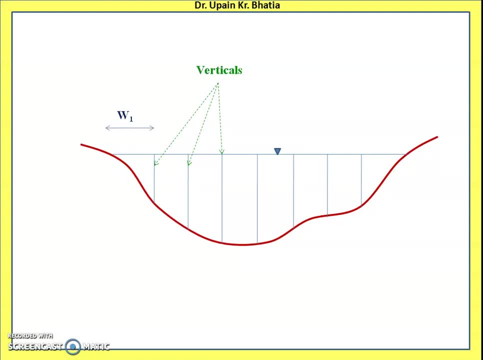 The distance of first vertical from the left bank is w1.. Distance of second vertical from the first vertical is w2.. Similarly, the intermediate verticals are at the distances wi and wi plus 1 from their respective previous verticals. The last vertical is at a distance of wn minus 1 from the previous vertical. 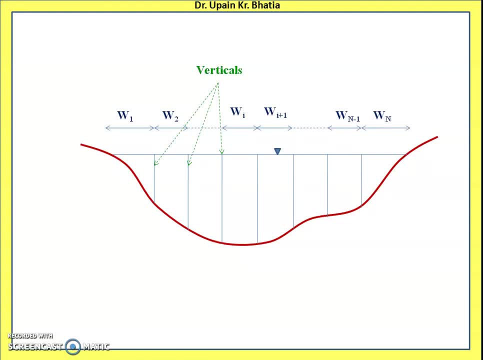 And the right bank is at the distance of wn from the last vertical. The red dot which has just appeared on the vertical line is the vertical line. The red dot which has just appeared on the first vertical is the point where we are going to measure the velocity. 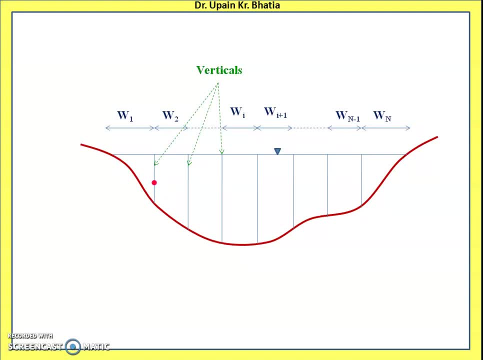 Either by current meter or by any other method. somehow, if you work out the velocity at this point, which is at 0.6 times the depth of vertical below the water surface, then the velocity at this point will be the average velocity on this vertical. 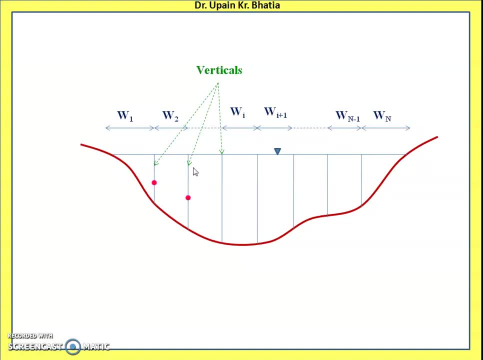 Similarly on the second vertical, this red dot. if it is at 0.6 times the depth of the vertical, then the velocity at this point again will be representing the average velocity on the vertical. If the depth of vertical is more, we can adopt two point approach also. 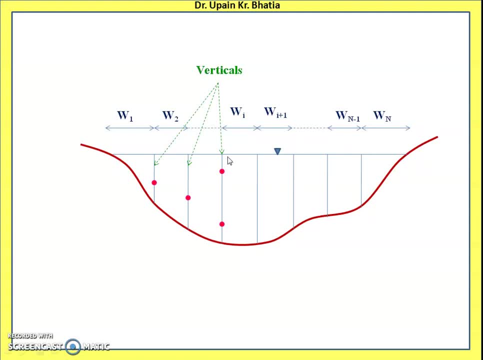 That means we have to measure the velocity at two points: First at 0.2 times the depth of flow and second at 0.8 times the depth of flow along this vertical, And average of these two velocities is going to give us the overall average velocity along this vertical. 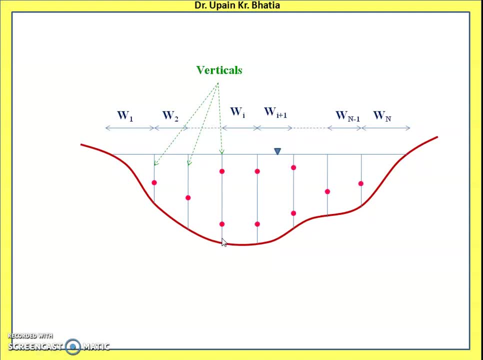 Similarly, we have marked other points also And after this we assume that we are having the average flow velocities along all these verticals. Now the next step is to divide the entire cross section into a number of segments using these vertical lines, the red dotted lines which are passing through middle of the two verticals. 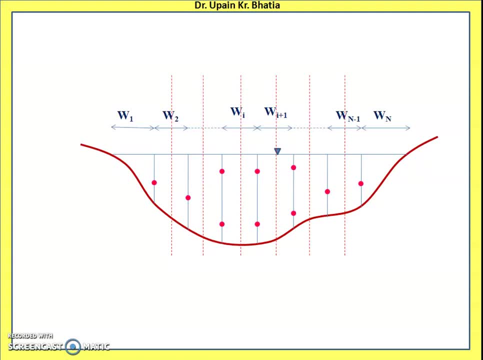 So they are dividing this overall cross section into a number of segments, Like: this is the end segment on the left hand side. This is the end segment on the right hand side, And the representative intermediate segment is shown in green color here And what you will notice is that every segment is having one vertical in the interior of it. 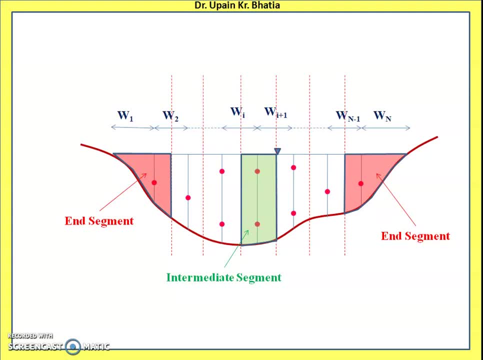 And we are having the average flow velocity That represents the flow velocity of this vertical. This is the segment. The effective width W bar for the end segments is worked out by using this formula: On the left hand side it is W1 plus W2 by 2, whole square divided by twice of W1.. 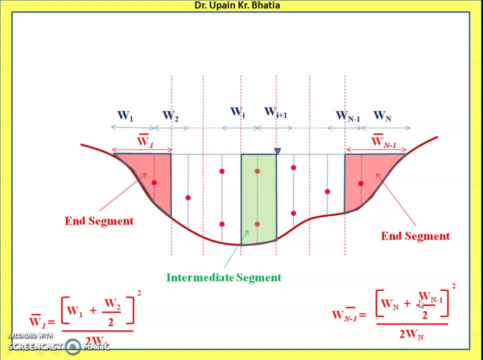 And on the right hand side similarly, it is Wn plus Wn minus 1 by 2 whole square divided by twice of Wn. For the intermediate side, the average width or the effective width of the segment is taken as half of Wi plus half of Wi plus 1.. 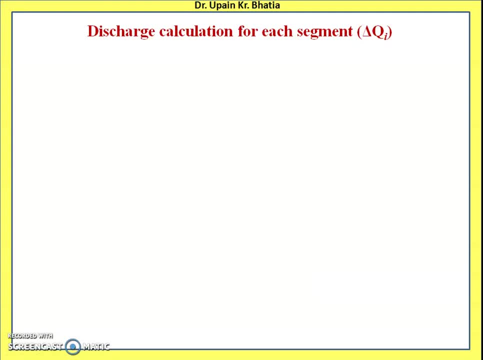 Now how to calculate the discharge through each segment. So let us consider that delta Qi is the segmental discharge, And this is equal to area multiplied by the average velocity Expanding it. It is. delta Qi is equal to W bar multiplied by depth of vertical, multiplied by the velocity of flow through the vertical. 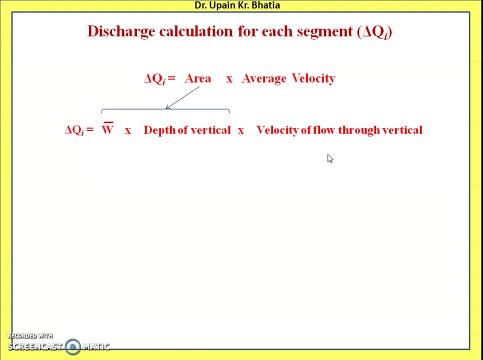 In this expression, W bar multiplied by depth of vertical is giving us the area of cross section of the flow, And the velocity of flow through the vertical is basically the average velocity as determined by the float or the current meter, And the total discharge through the stream is taken as the sum of 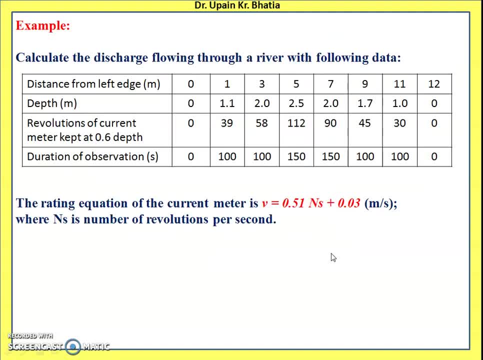 All delta Qi values. Here is the example: We have to calculate the discharge from flowing through this river from the following data, And the data is that distance from the left edge is given from 0 to 12 meters And depth of all the verticals is mentioned from 0, 1.1, 2, 2.5, 2, 1.7, 1 and 0 again. 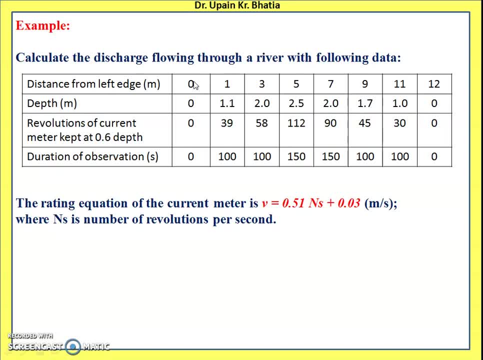 So this represents that the distance 0 and 12.. They are representing the extreme ends of the river, That means the two banks. Now for working out the velocity of flow. Number of revolutions of the current meter are given at 0.6 depth. 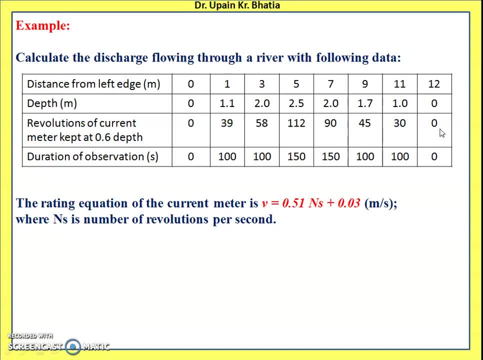 All these values are given as the number of revolutions for the current meter And the duration of observation is also mentioned in the fourth row To calculate the velocity of flow. The rating equation of the current meter is also given, as V is equal to 0.51.. 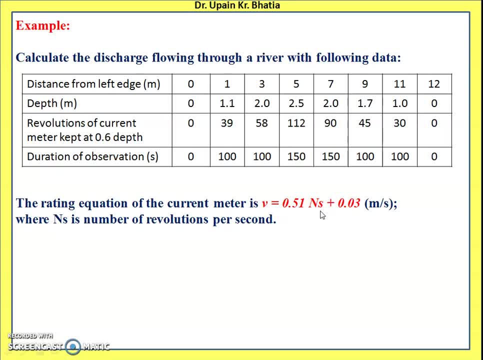 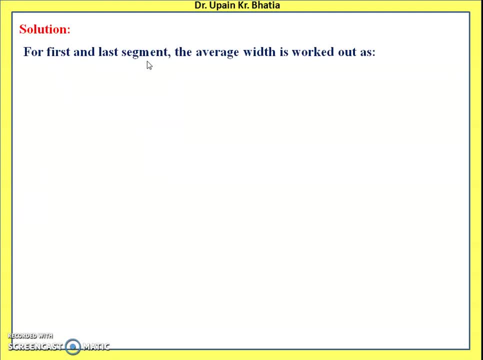 NS plus 0.03.. NS: here is the number of revolutions per second. So first of all we have to calculate the first and the last segment. The average width of these segments is: By using this formula, it comes out to be 2 meters. 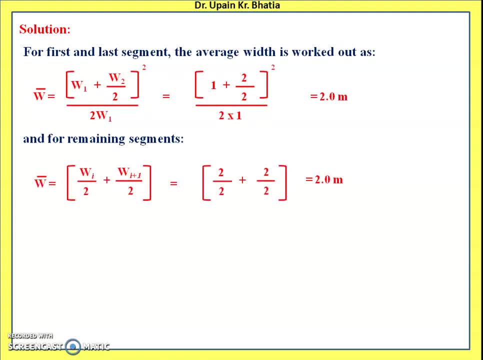 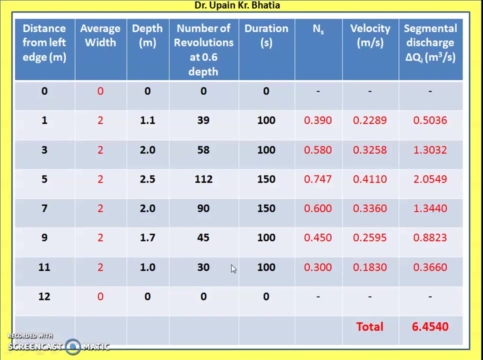 And for the intermediate segments We have to use this formula. Again, it is coming out to be 2 meters, Since the velocity is measured at 0.6 depth. The measured velocity is the Average velocity along that vertical, And the calculation of the discharge are presented in the tabular form. 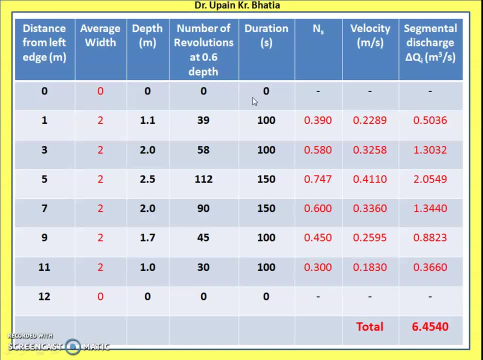 In this manner. Here the black columns Or the text written in black is already given to you. This is the given data, And red entries are Incorporated by us, So like the distance from the first, From the left edge, is given. 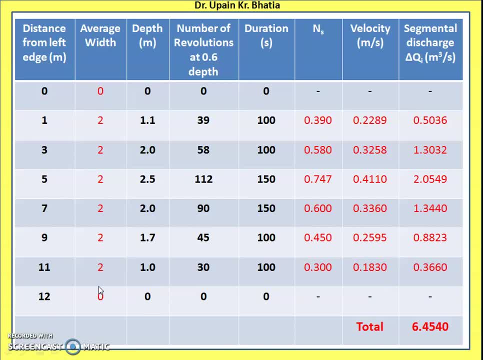 And the average width is worked out That we have calculated in the very first step. Then The number of revolutions per second is calculated As the number of revolutions recorded Divided by the duration in seconds. So likewise this entire column is worked out. 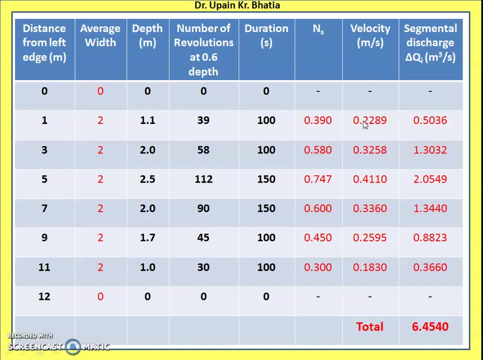 Then putting this value of n as in the rating equation, We can work out the velocities. So all these values of velocities are worked out And Velocity when multiplied by the area of cross section, Which is equal to average width multiplied by the depth. 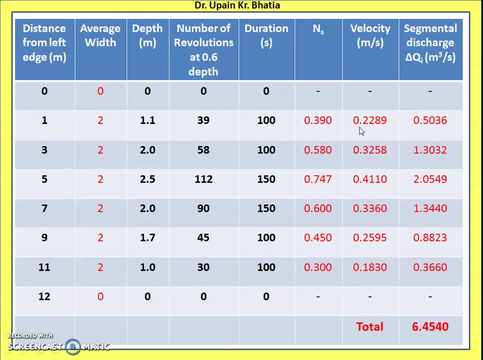 So this second column, The third column And this velocity column, If they are multiplied together, We are getting The segmental discharge delta qi From this particular column. So all these values are representing The segmental discharge through various segments. 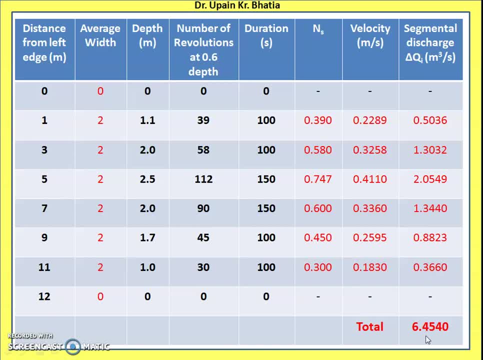 If you add them together, You get the total discharge flowing through the stream That is 6.454 cubic meters per second. So this way I think you can easily work out The velocity and the discharge going through the stream. Thank you.